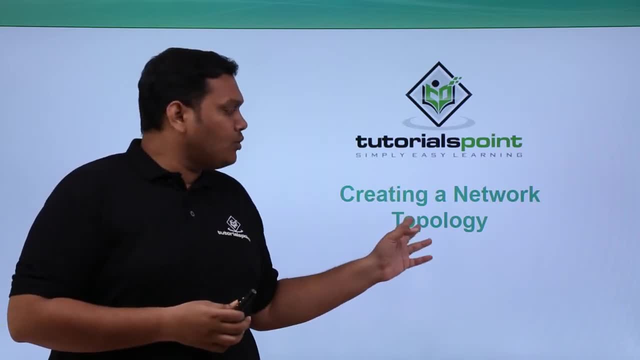 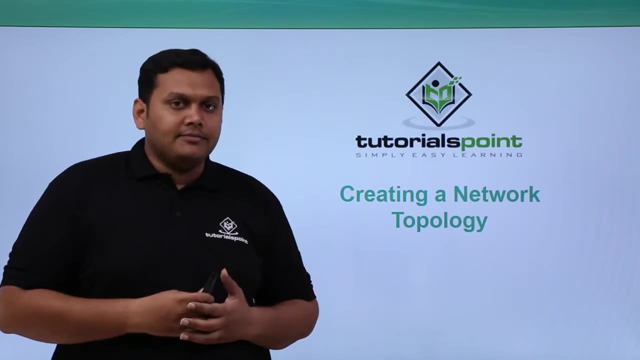 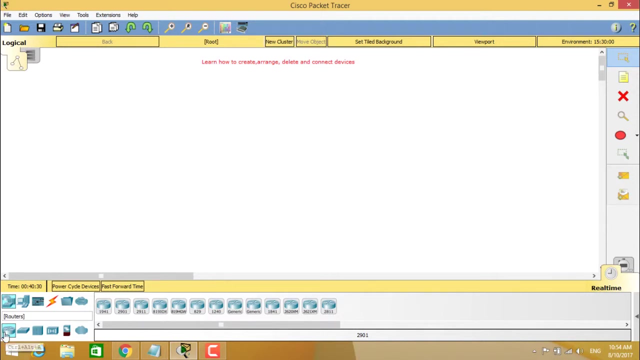 In this video we are going to discuss about how to create a network topology and for creating network topology, what are the steps required? we will be looking into it practically. So you see here, when you select this network devices thing, you see under that you have routers, you have switches, you have hubs, you have wireless devices, you have security. 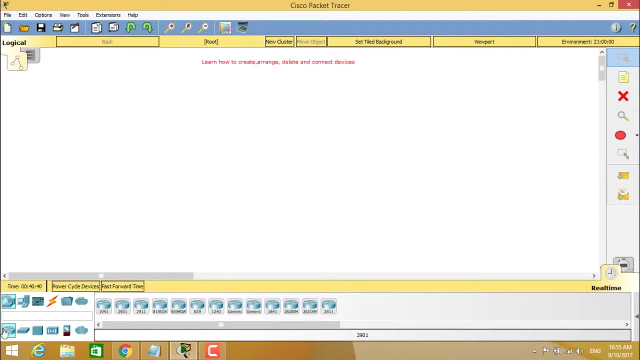 devices, as well as WAN emulation also. So when you select each of this router, you have the number of types of routers available here. When you click on switches, you have the generic, the series of switches also available, including the hubs and wireless devices, security and. 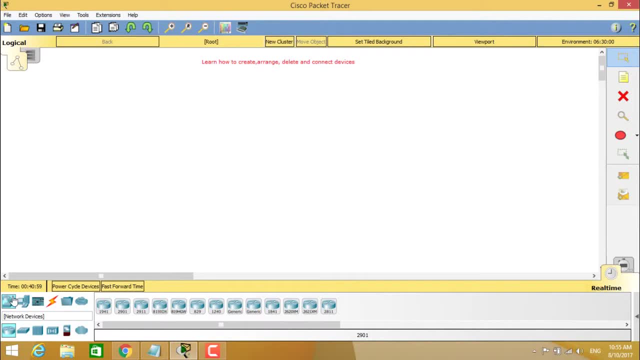 also about the WAN emulation. In the same way, when you select this end devices, you see, under the end devices, the first one is computer, laptop, computer, computer, computer, computer server. you see here printer, you see iPhone, that IP phone, which is VoIP device as well as phone. 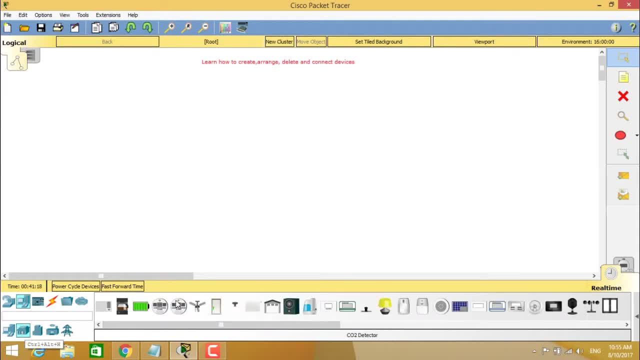 TV etc here and also you can see there are many options. so like appliances, AC battery and CO2 detector etc. In the same way, in the smart city- you can see here the ATM pressure monitor battery, you can see CO2 detector, you can see fan etc also available. So we'll see how to create. 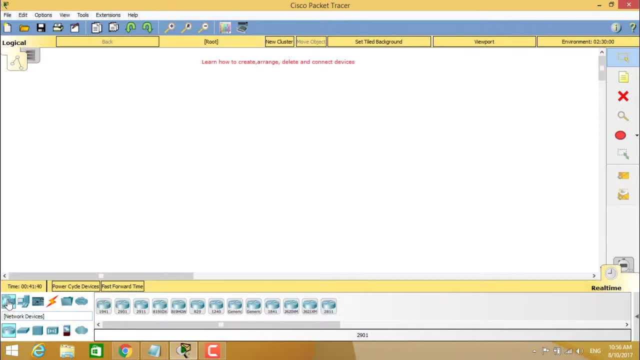 a range of network topology of the network. So here in the smart city, you can see here the ATM pressure monitor battery, you can see CO2 detector, you can see fan etc also available. So we'll see how to create a range, delete and also connect devices among these. first we go into the network devices and we select the. 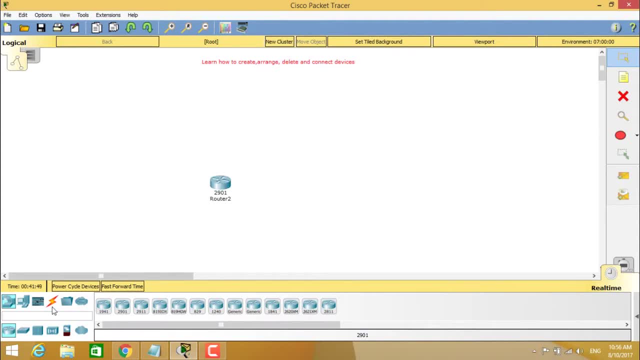 one type of a router here. so to select that you have to, you can do one thing, like you can click on this, the series of router you want, and you can click on the, the panel which is available for us to place the workspace, so you, when you wanted to delete any selected item, you can select this. 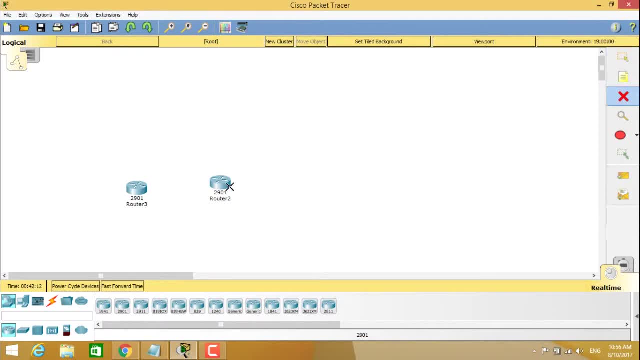 into cross on the right side pane so that it will be deleted when you click on it again. go into the selected pane and now we have selected a router. so now we'll go with the end devices and from end devices rich to a generic pc. so, apart from this pc, now we will select this. well, we will. 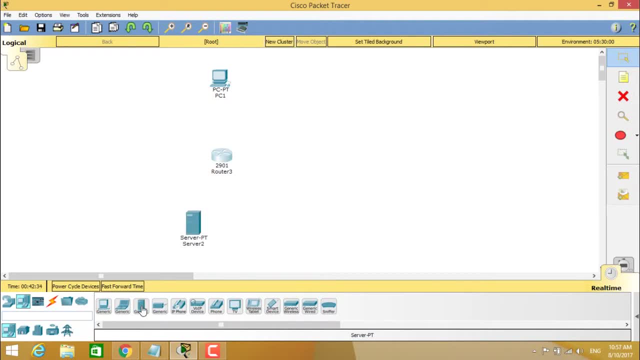 be selecting here as different to rrade objects and we will go. and we received our access right, the generic server, so we will take two generic servers and a router here, which is which is placed separately beside now. we wanted to select a switch also, so go to network device under switch. 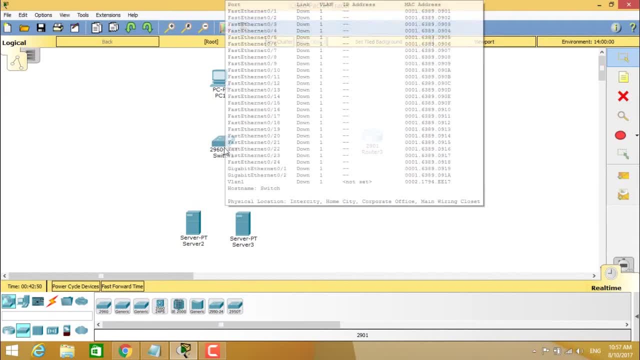 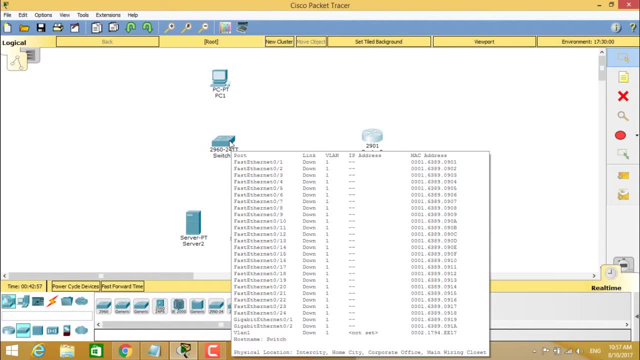 we'll go with 2960 series of switches here and you see, when you place on this, you can clearly see what are the ethernets available here and what and the state of that, and also under which virtual and they are available, including the mac addresses available. these are auto generated because this 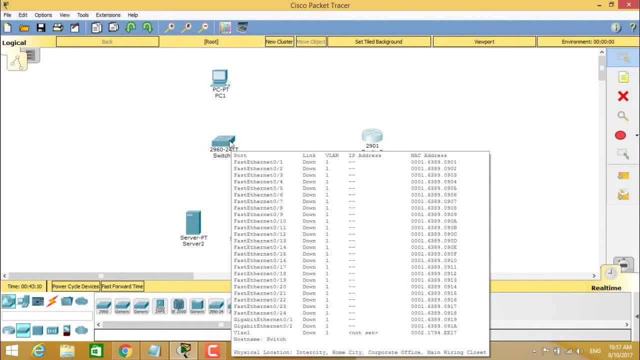 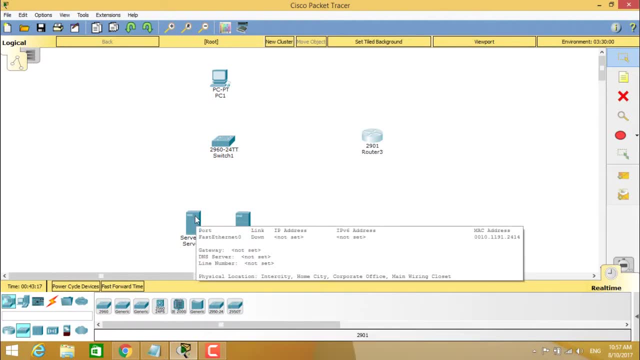 cisco packet tracer is a simulated virtual environment so that it is auto generated. so, coming to the server, under this server you have fast ethernet zero. it is clearly given only one fast ethernet is available here. in the same way, this other server, three, also has the fast ethernet zero which is in the down with the mac address available. 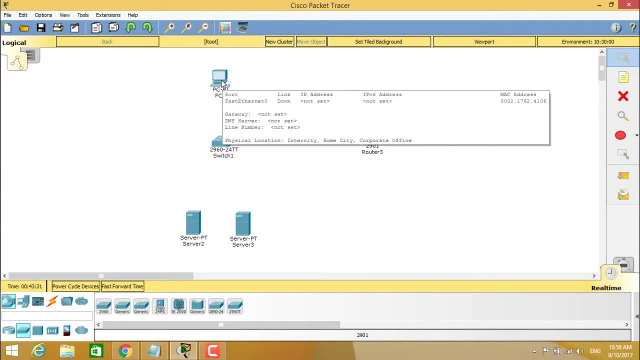 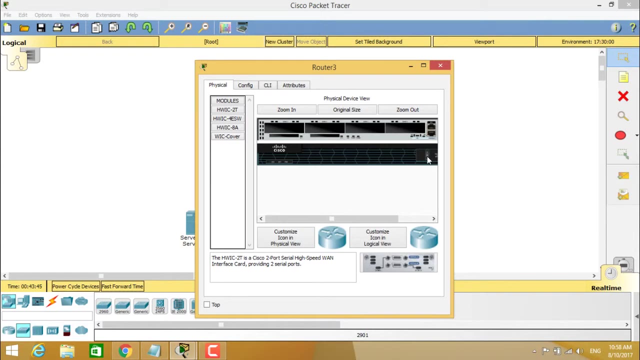 so coming to the pc, so this pc has fast ethernet and zero and it is also having a mac address associated with it. so now automatically in the cisco packet tracer the routers are in the on state directly so that you have to off it and also you see here there are no modules available here. 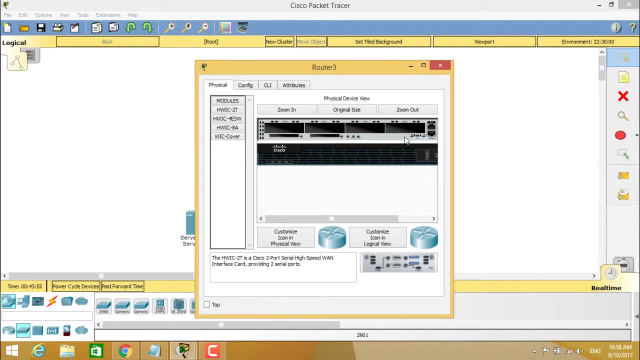 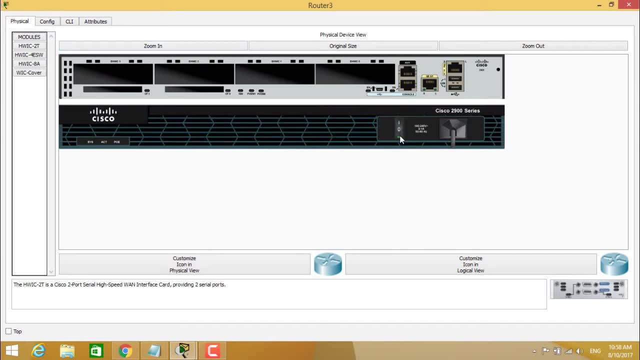 so we have to assign a module to the cisco packet tracer and we have to assign a module to the cisco packet tracer, assign the modules only in the powered off state. so that's the reason you can see here clearly that if you zoom in you can see here there is an option called power on and there is an option. 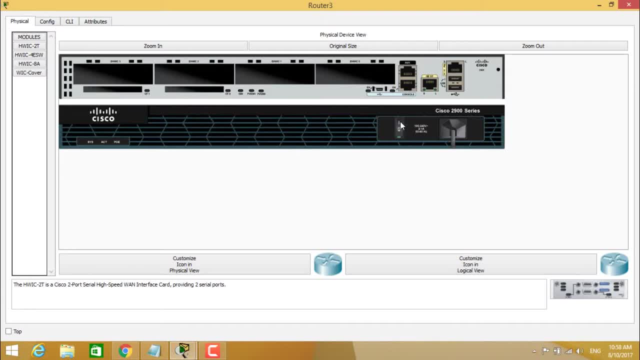 called power off here. so by default, when you double click on the routers configuration window, automatically this- the router will power on. so this is power on symbol. you see the green green light here. so we have to power off and we have to assign the modules here. so we are assigning this module. clearly. you can see how i am dragging and dropping. 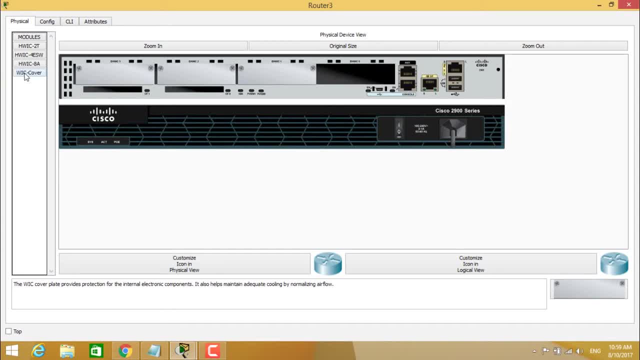 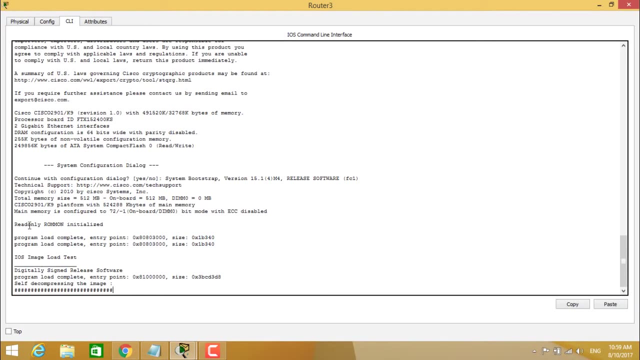 and you can also clearly see. apart from the wic, you can also assign hwic 2t, also available here. now you see, the modules are arranged here and now you can power on the router. so this is how happened and you can see here clearly that read-only rom monitor has been initialized. 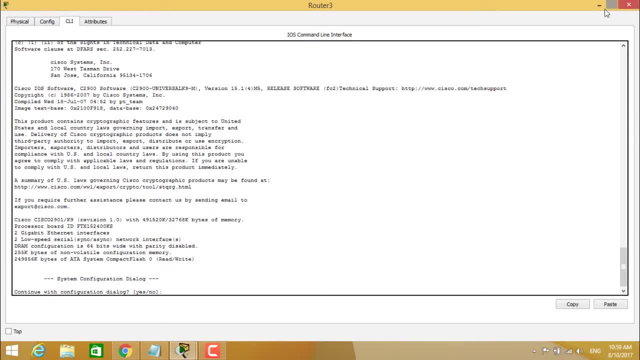 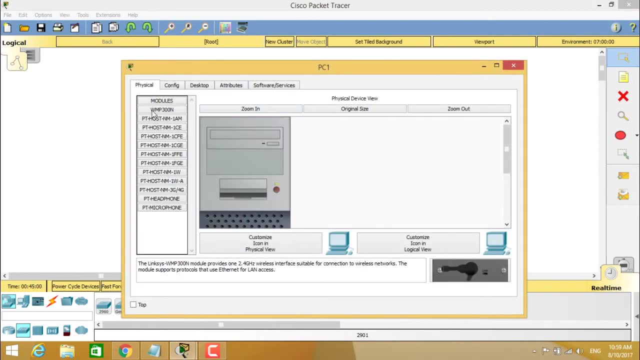 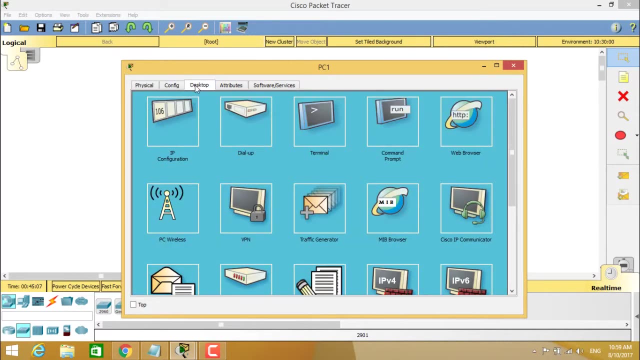 and you can see again. it got started okay, and this is about the router and you can see clearly about the pc connecting to the p. the pc is also having the modules available and this is the tabs available under pc, which is desktop version: dial-up, ip configuration, terminal, command prompt, etc. and coming to the attributes, it is given. 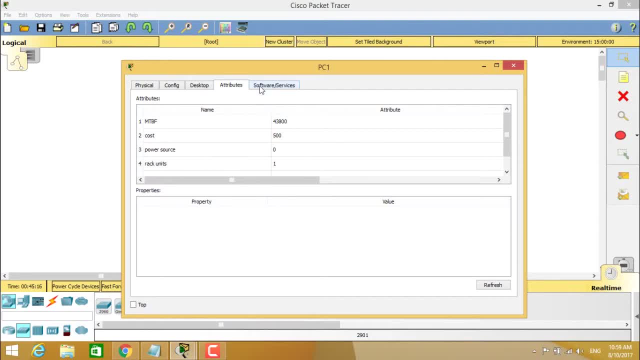 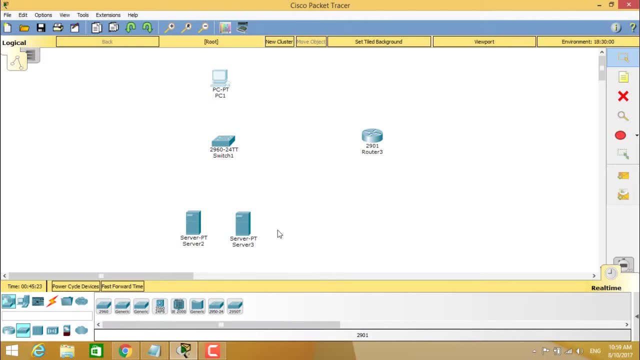 clearly the simulation attributes available and the software services available for the pc. so now we want to create a network topology, so we have to go with. this is called connections and you see, this is automatically chosen connection. so for every connection there is an, there is a name. 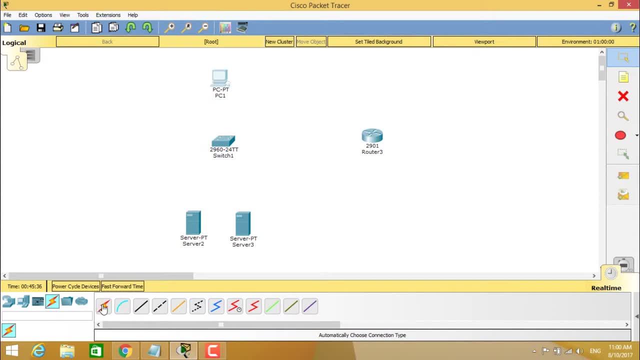 you can see the name details here. clearly. this is automatically chose connection type. this is console cable, this is copper straight through cable, this is copper crossover cable, this one is fiber cable and this one is phone cable. this one is coaxial, this one is serial DC, this one is serial DTE. 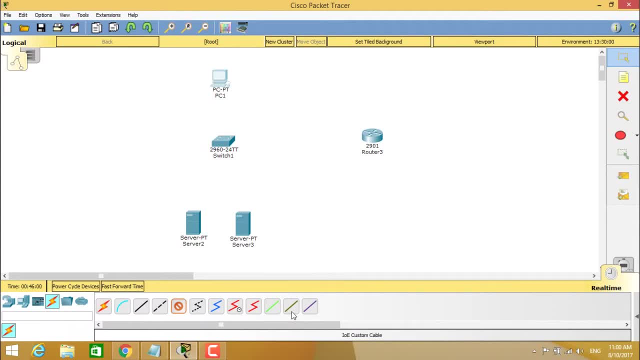 this one is octal cable, this one is IOE custom cable and this one is USB cable here. so now we wanted to connect our PC to a switch and to the two servers, server 2 and server 3. so for that we have, we are selecting this cable, which. 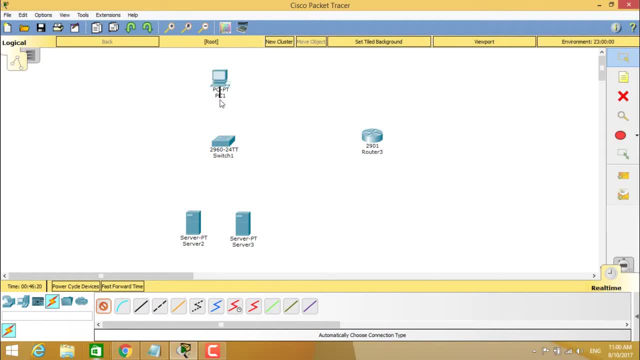 is automatically chosen connection. so here we are connecting to the switch. so from switch again we are connecting it to one of the server again here from the switch we are connecting it to other server here. so you see, here the PC is now connected to a switch, to a server. this is called, and now we are connecting. 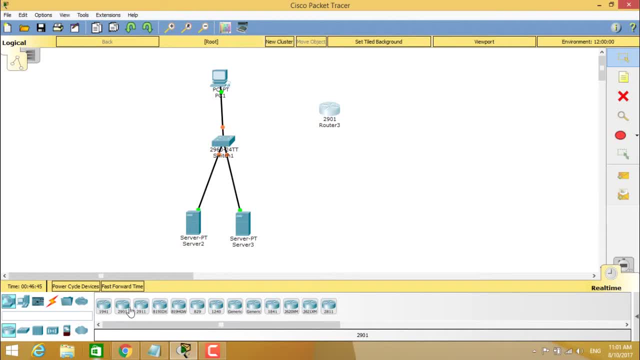 for three routers. so we go to network devices. we have chosen the other router and we also chosen the other router. and now for this router we have to select the connections, which comes under the c, serial, dte, and here we are connecting to serial port, to this gigabit ethernet port. and you see, here the compatibility issue has erased that the cable. 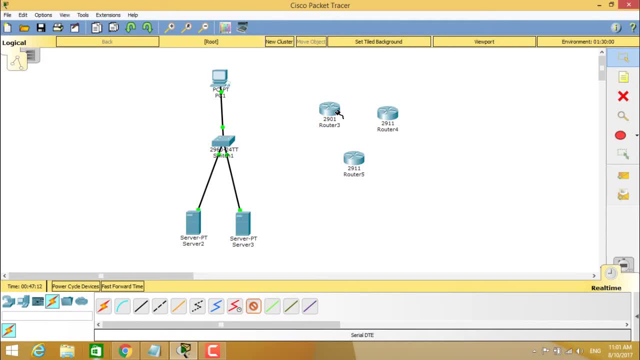 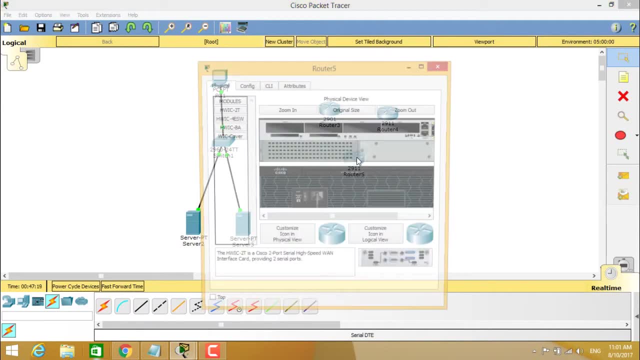 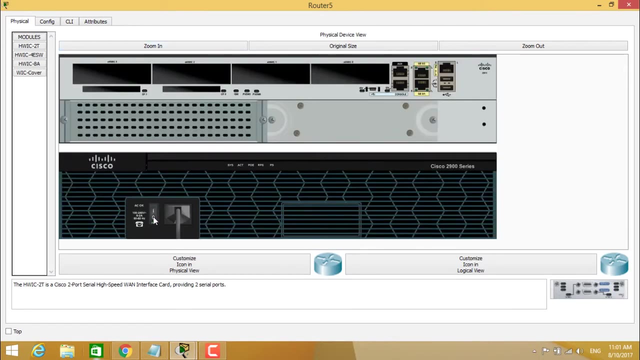 cannot to be connected because we are connecting it to serial port, to the gigabit. it has the serial available. so now we are coming back and now you see, here we are configuring it again back because, you see, the modules are not arranged so that we are powering it off. we are assigning the modules. 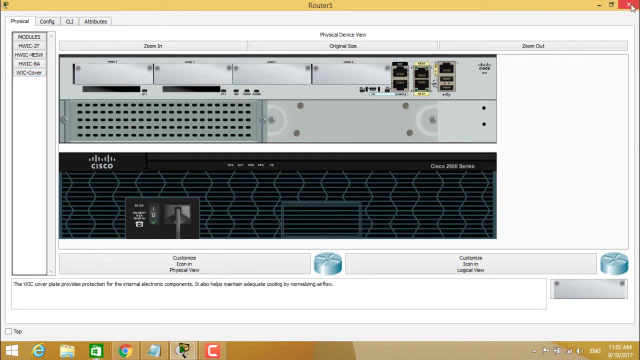 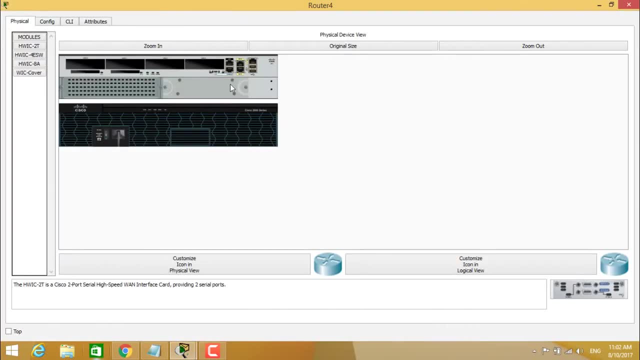 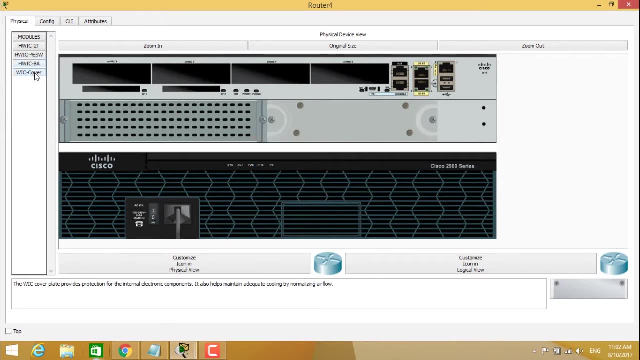 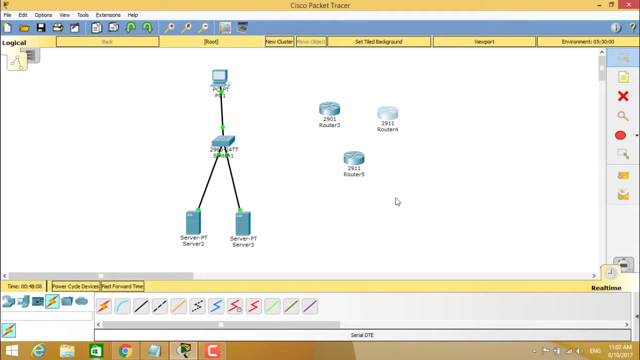 after assigning, we are powering it off, and now it's powered on back. the same way with the route of four also, and we have powered back again the router. so here, if you check clearly, that the green symbol indicates the connection has been established correctly. so now we have chosen. 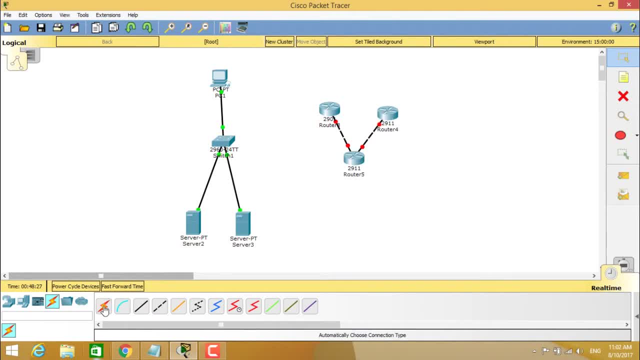 the automatic choose connection type. and now we are connecting this one to one printer. so, coming back to the end devices, acking internet connection can be connected to another computer or same. remember after which equipment we connected this pin to the virtual circuit and now connecting this router to this printer. and now this switch should be connected to the router so that we have choosing automatic choose connection. so now this: this is a network to terminal connection in the software. you are not cutting here your plug and draw connection. short connection connection in the software: connectnego on the internet background. you are not connecting connect, you are not connecting to the next to existing selectednetworkальное. 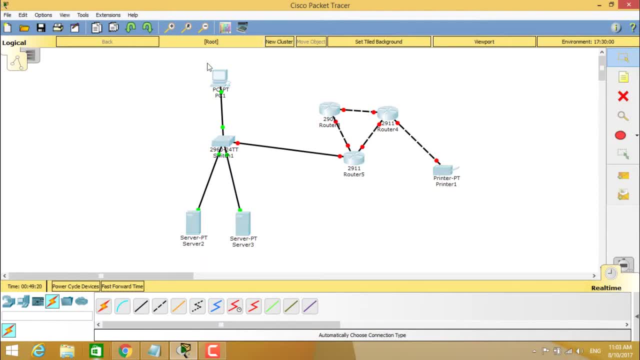 available if you check clearly that the PC is connected to a switch to the servers and the switch is again connected to three of the routers in the same area and also in the same configuration, and now this router is connected to the printer. so this is called network topology and, if you want, 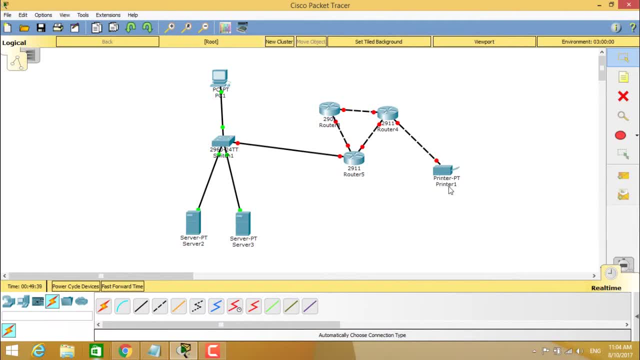 to delete any of the connection you can see. you have to select this into cable and you see this into is for deletion of the devices you can select on it automatically the connection will be deleted in the same way. if you want, if you don't want one of the router to be available now, you can connect this.